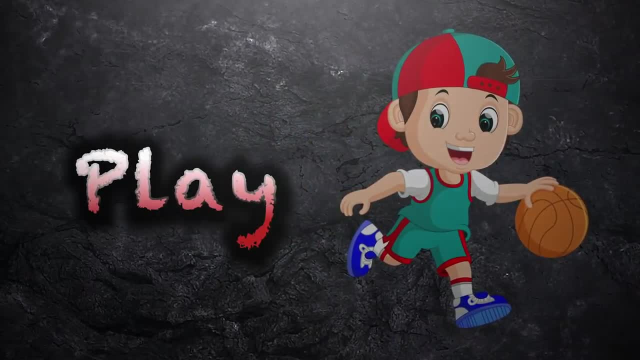 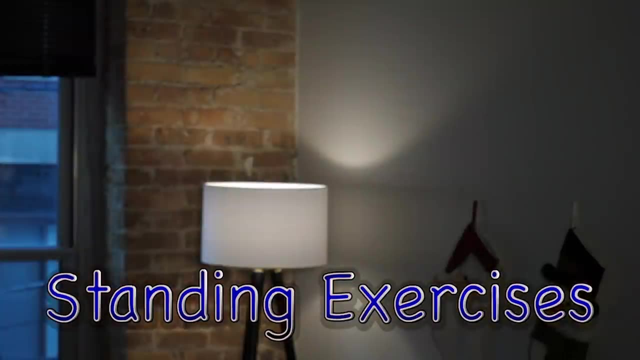 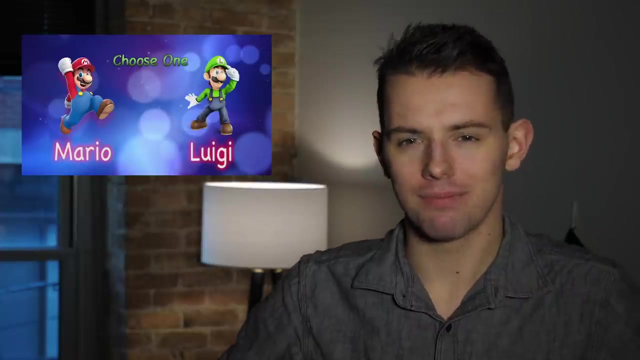 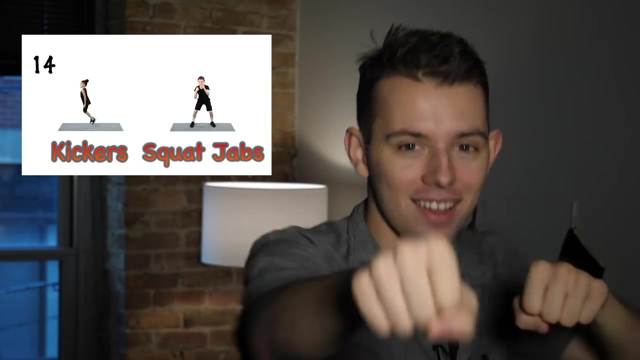 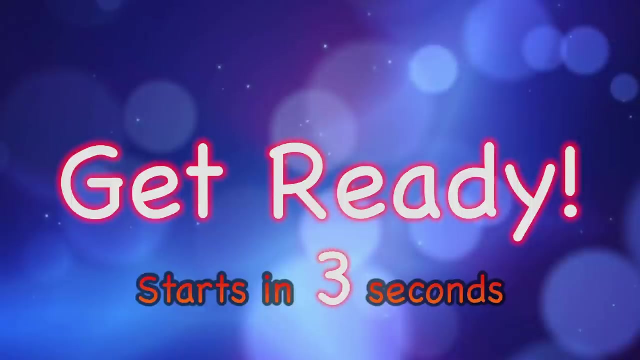 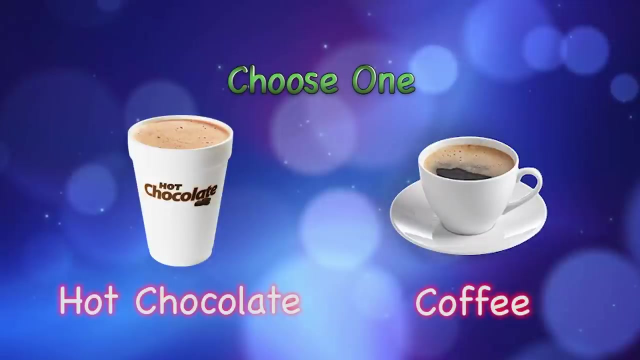 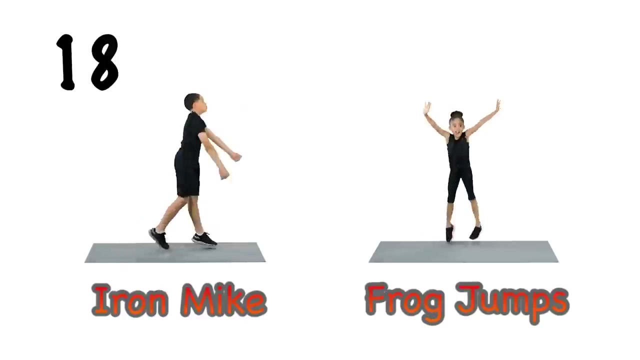 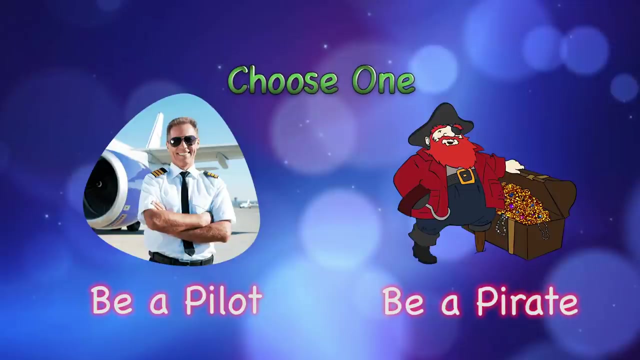 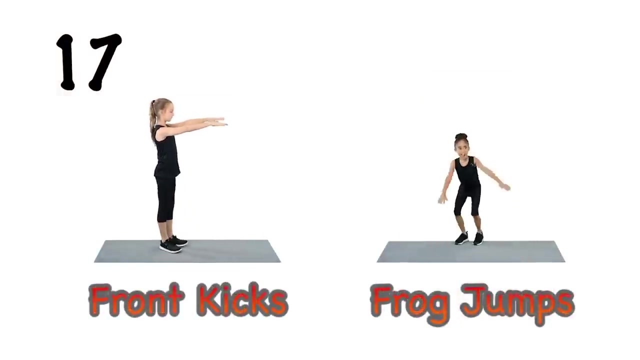 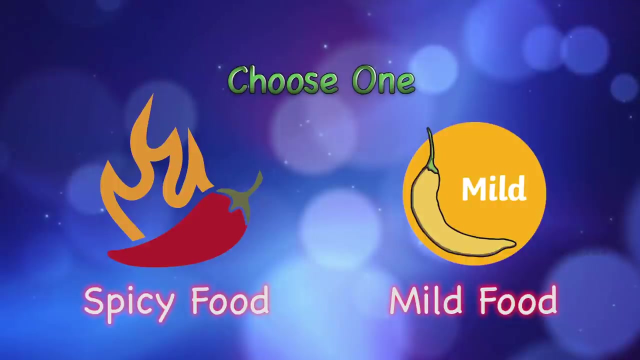 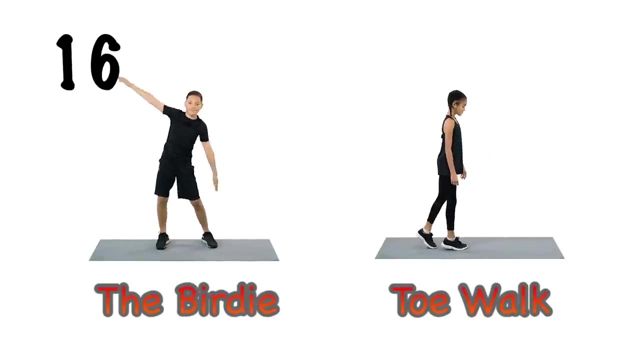 All right, so do I like Mario or Luigi? It's got to be Luigi, All right, looks like I'm doing the squat jabs, All right, let's go. All right, let's go. All right, let's go. 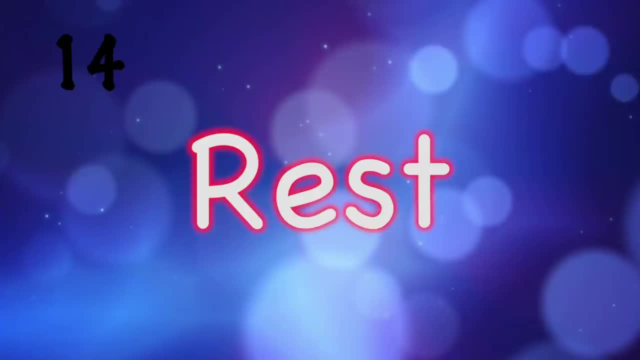 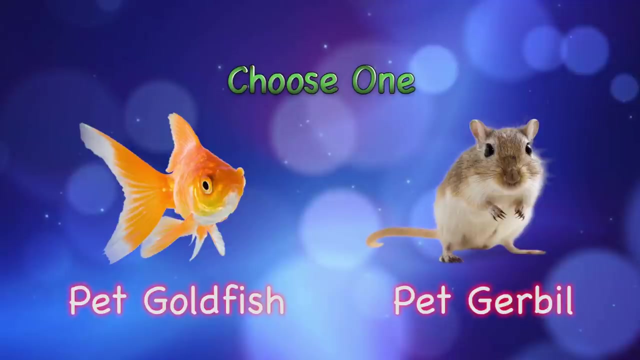 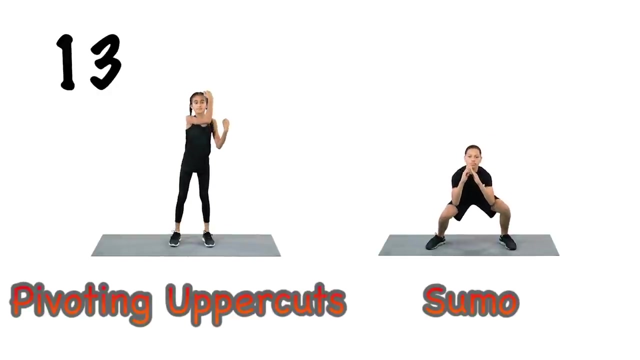 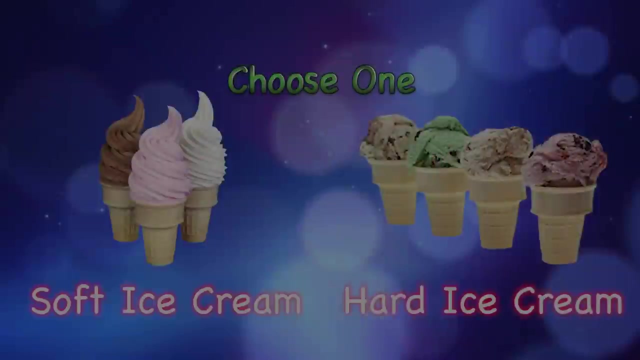 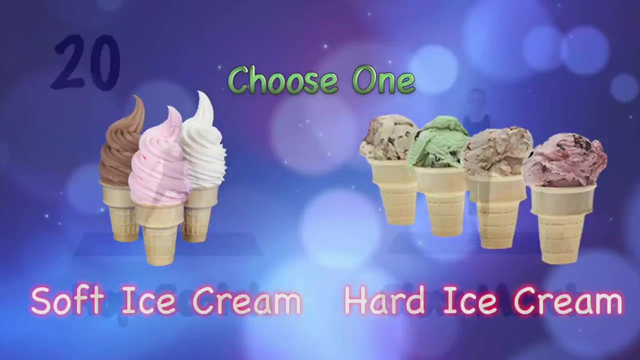 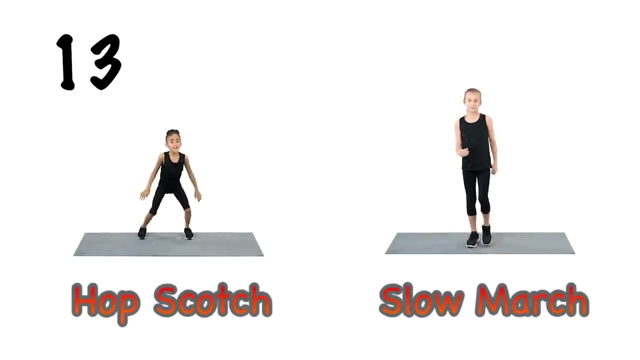 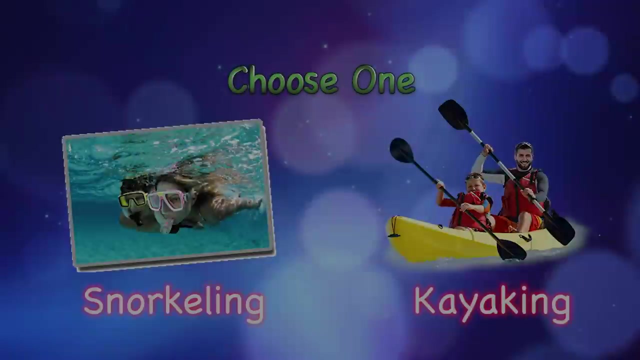 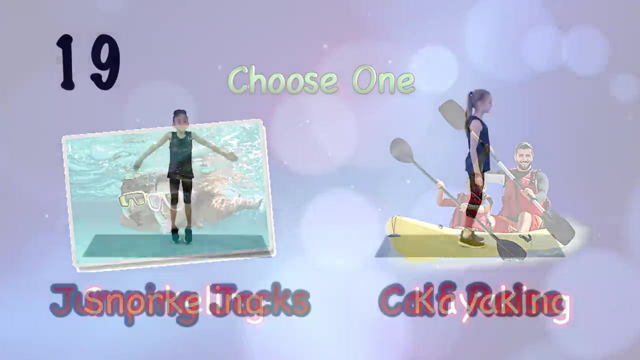 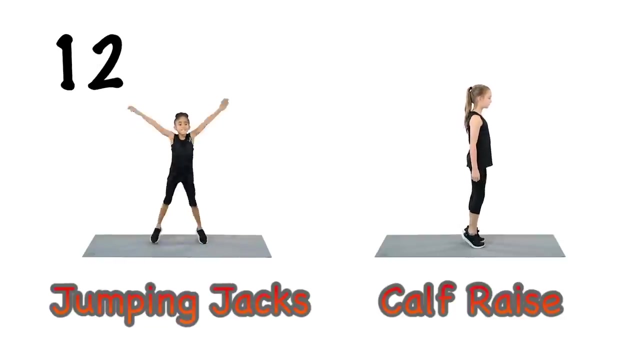 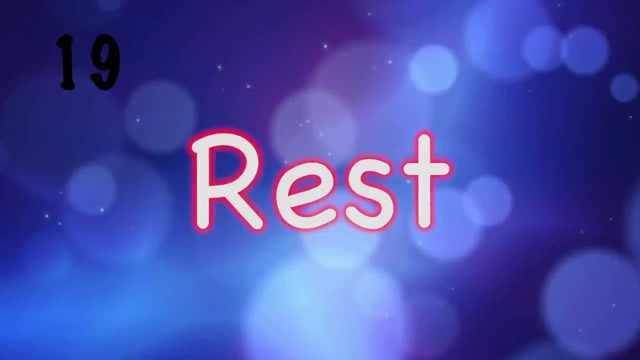 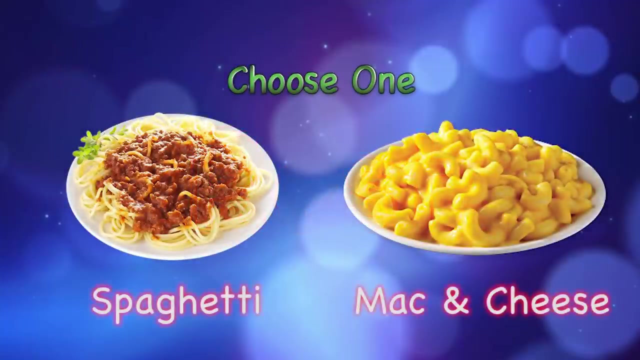 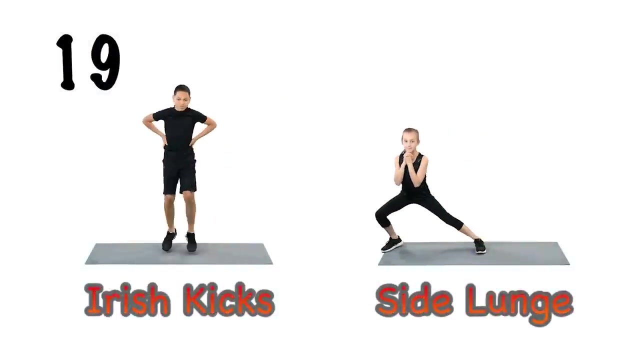 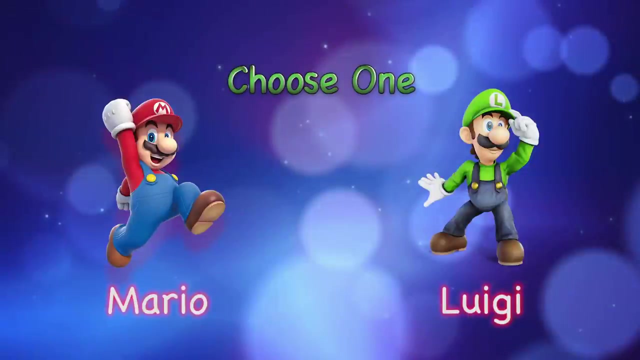 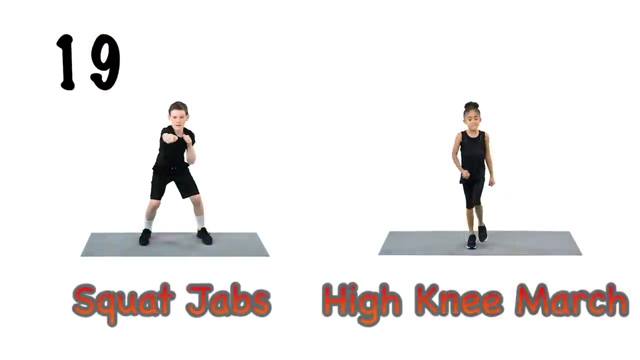 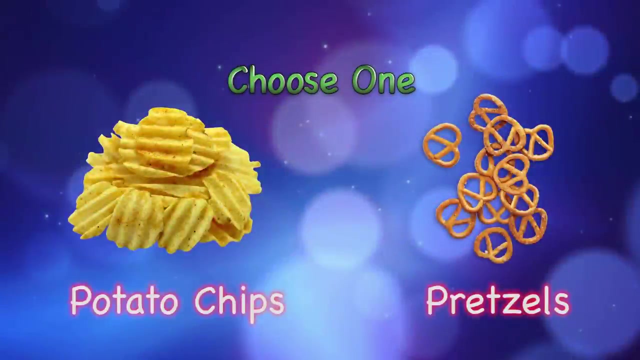 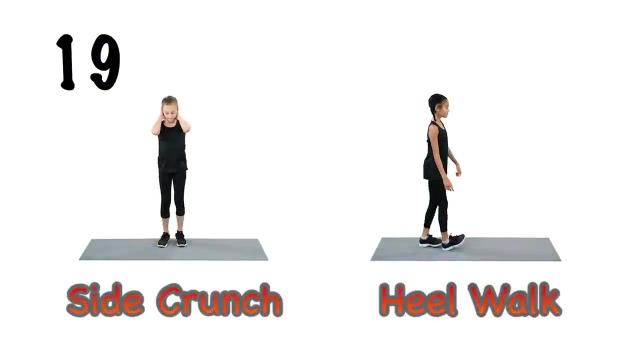 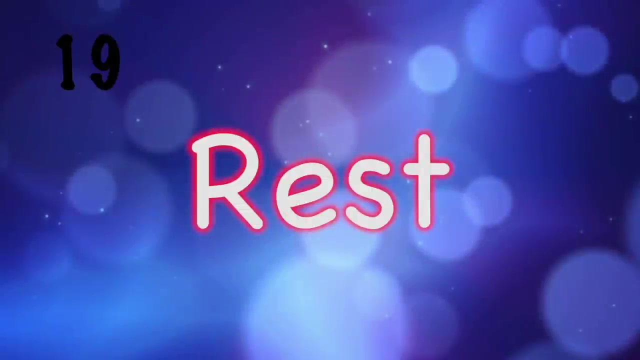 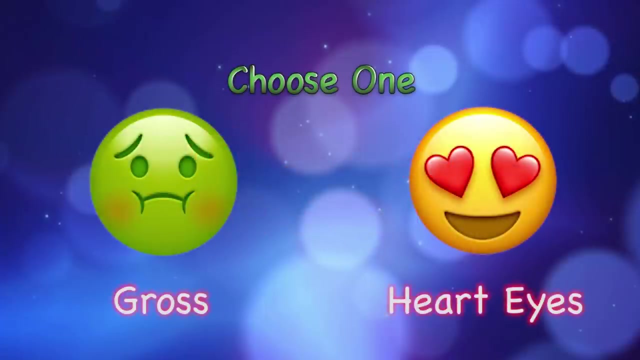 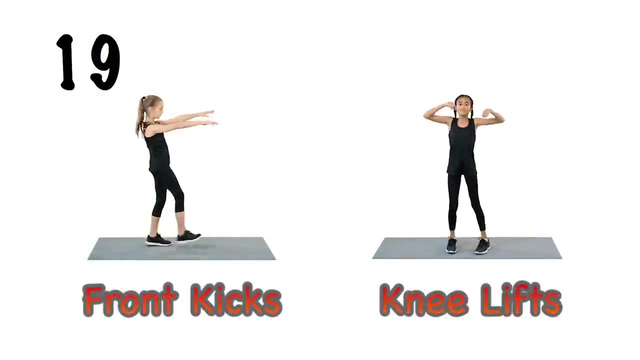